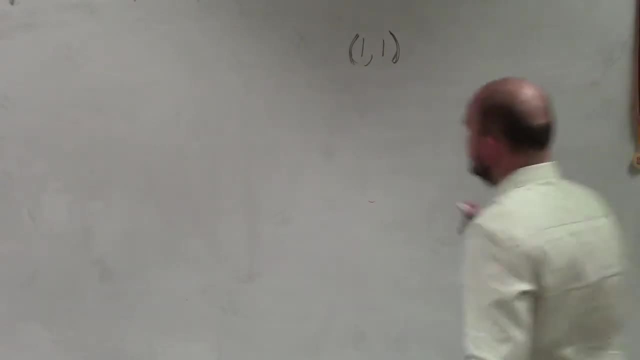 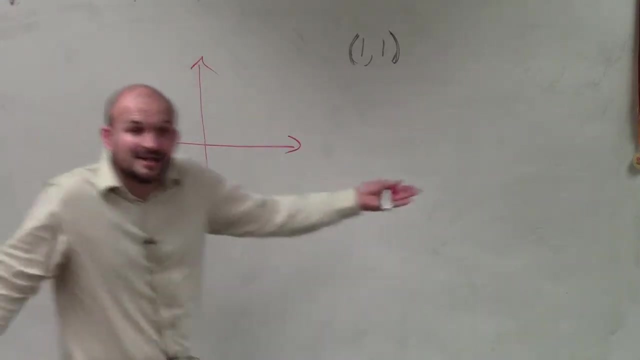 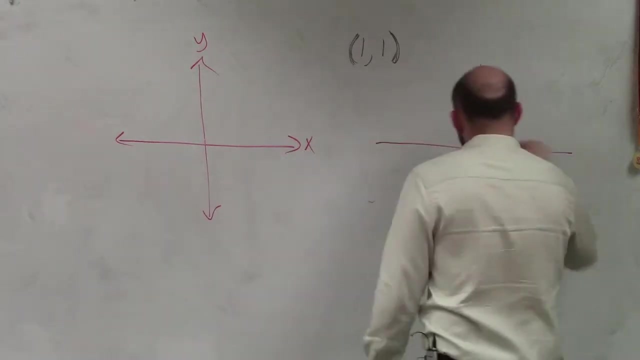 So it says she's just a friend, All right. When we're looking at this again, it's an x and y coordinate. We want to convert to polar right. We want to convert from x to y to this crazy thing right, Where this represents our r, and here's our thetas, which. 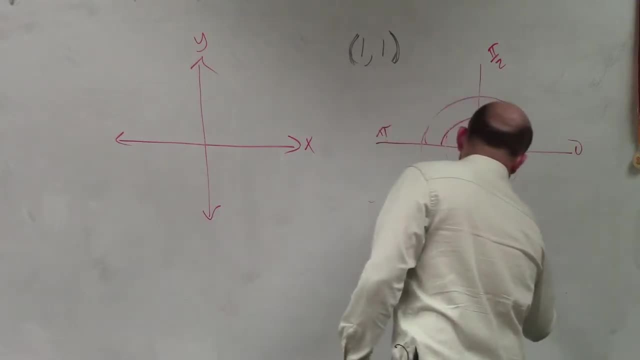 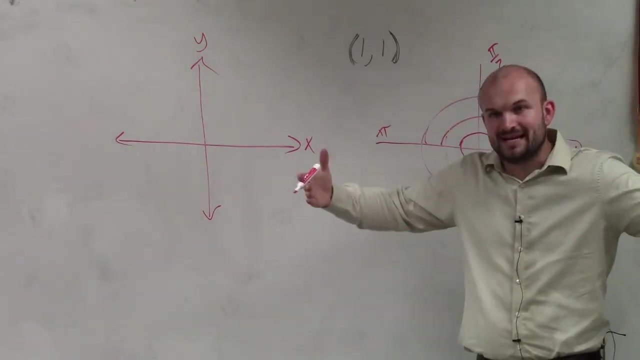 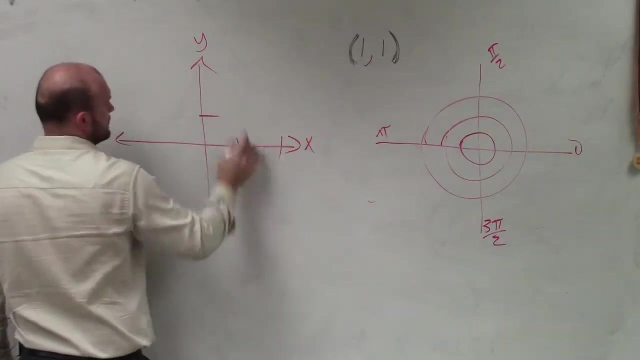 have zero, pi halves, pi, three, pi over two. So one thing that might be helpful, ladies and gentlemen: when we're using this, we're concerned about the radius, which is the hypotenuse and theta. So let's graph one comma one. Actually, let's do it even bigger: One, one. 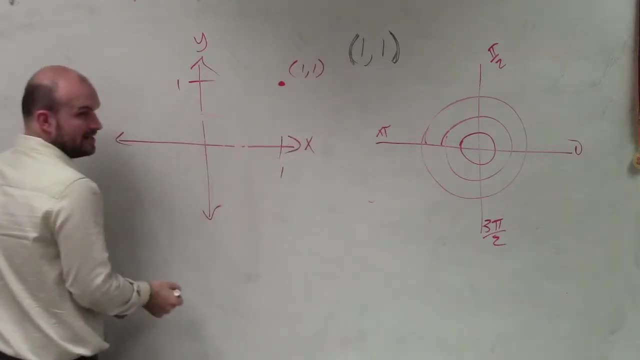 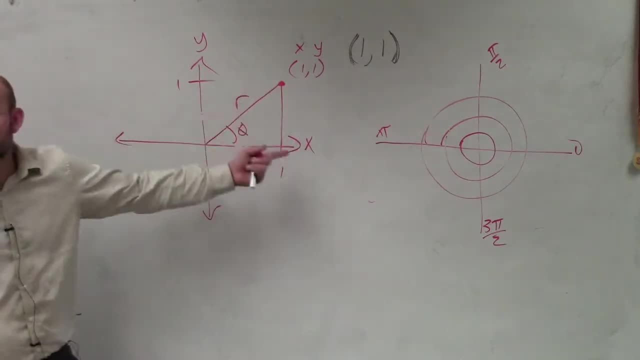 concerned about knowing what r is and what theta. R just represents the radius. It's also the hypotenuse of this triangle. So, knowing that this is one and that's one and that this is a right triangle, can we figure out what r is? Of course we can One squared. 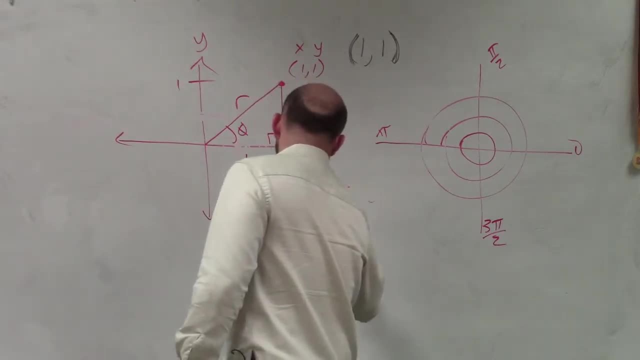 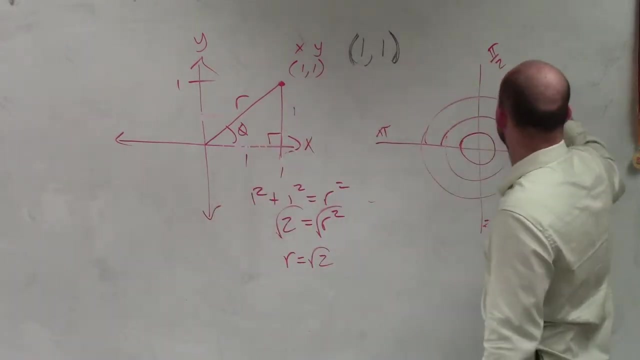 plus one squared equals r. squared Two equals r squared square root. square root R equals the square root of two. So when I want to convert this, I'm going to have: r is the square root of two is going to be somewhere in between one and two, right, Whatever it might be. So 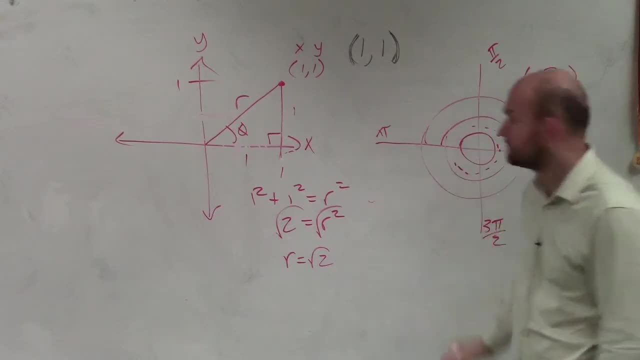 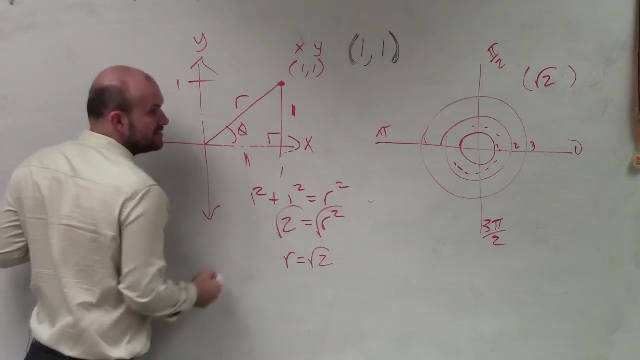 it's going to be somewhere around this little. I'm going to make a makeshift ring in there. Now we need to be able to figure out what theta is Again. the only thing we know is the opposite side and the adjacent side. So we can say: tangent of theta equals one over. 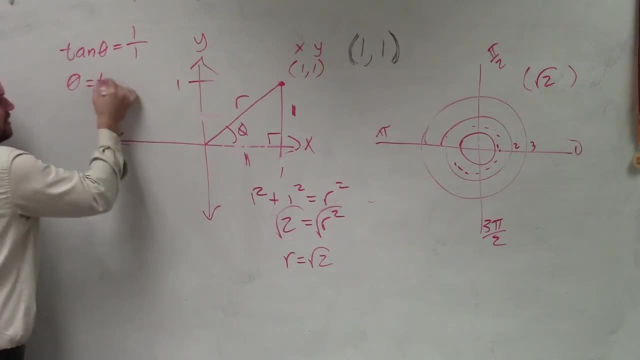 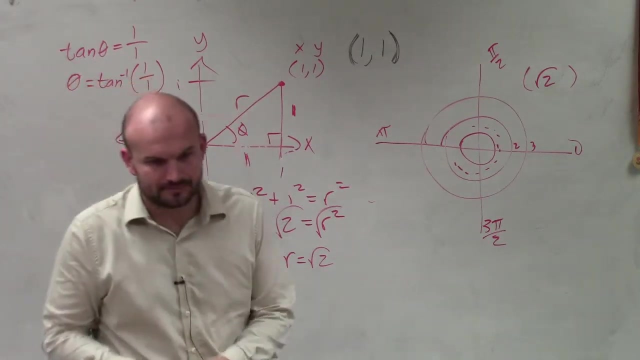 one. So, theta, my angle is equal to the tangent inverse of one over one. So now I take my left hand and I take my right hand, and I take my right hand, and I take my left hand and I'm going to do a lovely calculadora And make sure that I'm going to be using